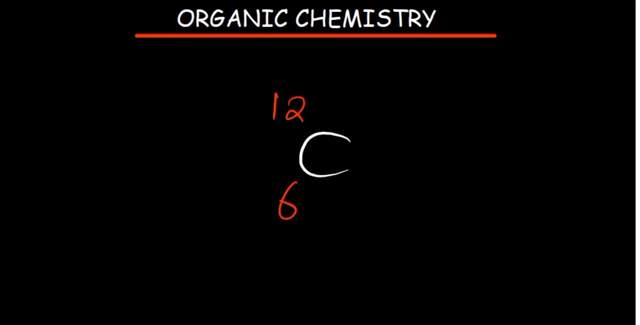 Okay, so a few things that we need to know about the carbon atom is, it has got an atomic number of 6 and has got a mass number of 12.. So, looking at the atomic number of 6, we are able to come up with what we call the electron configuration. 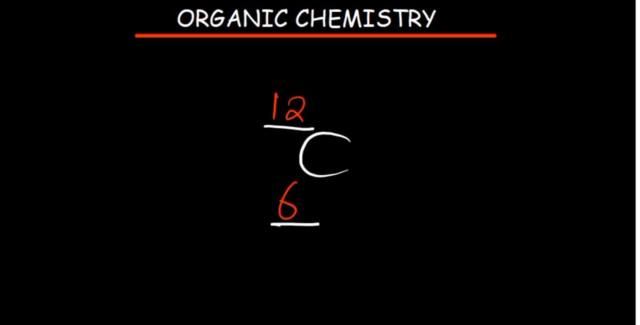 And of course a basic electron configuration would be: we have how many electrons? We have 2 electrons and then followed by 4 electrons, right? But using the orbitals we can also write the required kind of electron configuration. So basically, we have 1,, 1s2 and then we have 2s2 and then we have 2p2, right? 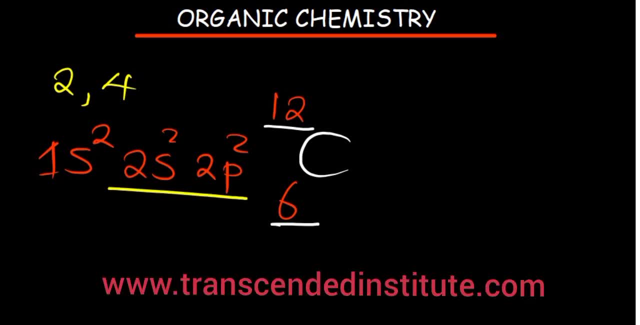 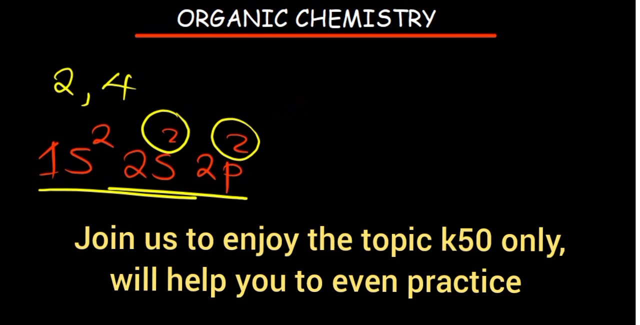 So we'll notice that in our outermost shell we have got 2 electrons in the s-orbital and 2 electrons in the p-orbital there. Okay, that's very important. So, looking at this, this is going to give us a kind of hybridization that we expect this carbon atom to undergo. 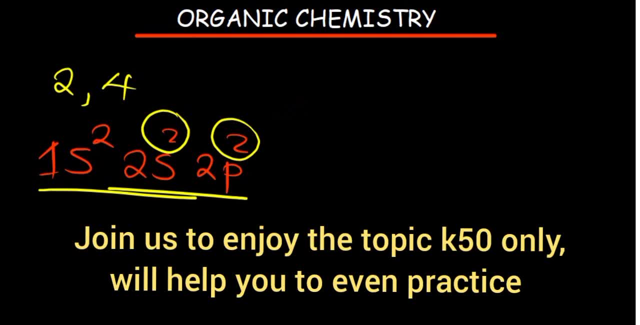 Okay, so, looking at a certain example here, So because of compounds that are made up of carbon, I can draw some of them and then we'll come up with a kind of hybridization that carbon is able to undergo. And, of course, one thing that is very important for us to note as we start is carbon forms a maximum of 4 bonds, because it has got a valence of what 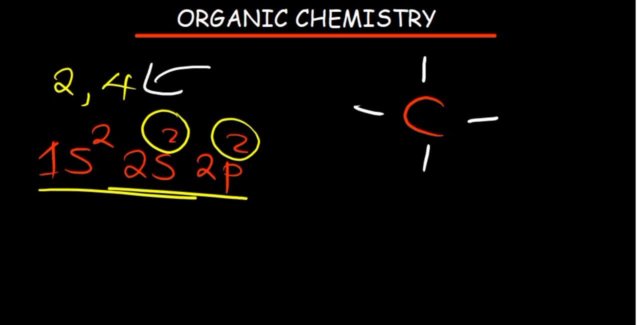 Because it has got a valence of 4.. So it's capable of forming a maximum of 4 bonds. That's very important. So every time we are drawing any compound containing carbon, we need to make sure that it has got it. 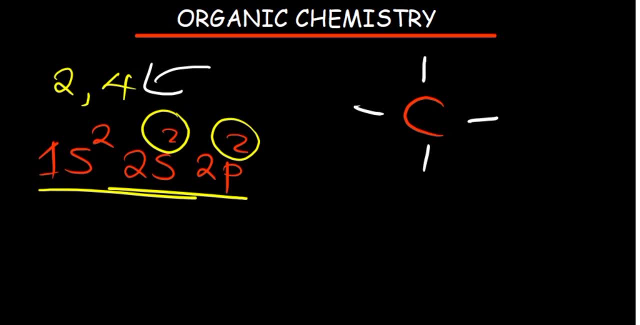 So basically 4 bonds. Okay, that is even going to help us as soon as we get to draw certain compounds. Okay, so I can draw this compound. I'm sure I've come across it. So this is carbon dioxide. Okay, I'm not sure we want the electrons. 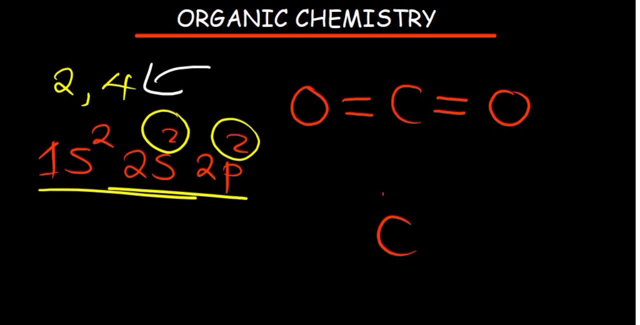 And then we can also talk about this kind of a compound And when we have hydrogens there, And then the other cases they can also talk about. Let's have this one Where carbon is forming single bonds- Yeah, So hydrogen hydrogen there, hydrogen hydrogen. 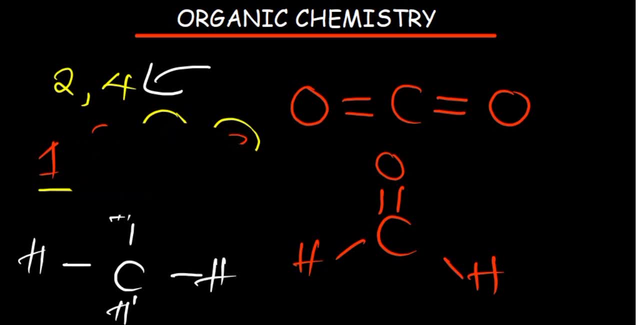 So so far we can see the different bonds that this carbon is able to form. right, And then one more that I can draw is where we have carbon forming 3 bonds and then a hydrogen there. Okay, interesting. So these are the different 4 ways in which carbon can actually react or form compounds or bonds with any other atoms, right? 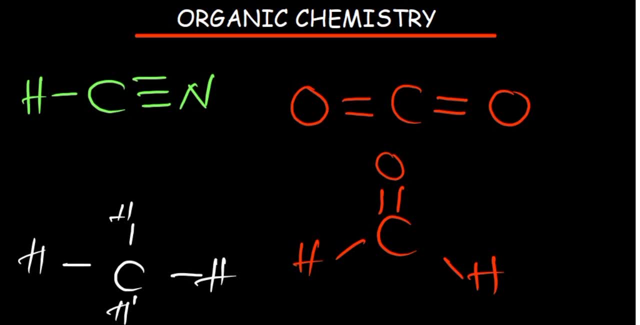 This is what we are seeing And, of course, what we are looking at is: where is the triple bond? So we can see that carbon has formed how many connections? Two connections right. So in this case, the kind of hybridization that is undergone, we can call it sp hybridized. 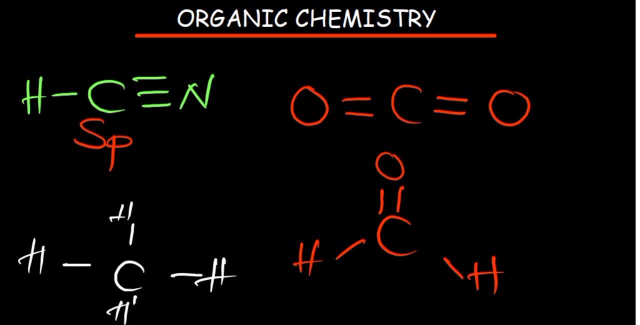 And, of course, the other cases as well, As you can see where we have carbon dioxide there. That is also sp hybridization. And then the last one on the left, This is sp3.. And then this is sp2.. So one easy way of you identifying the kind of hybridization that the carbon has undergone is by counting the number of connections. 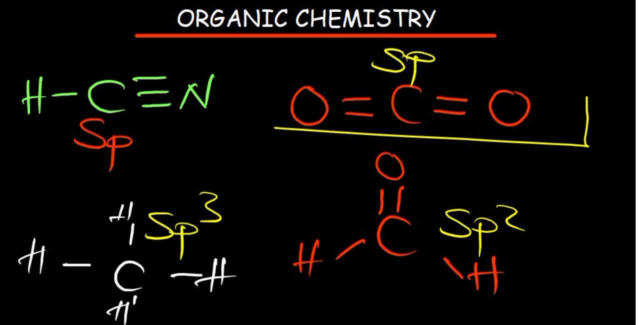 And in that case you get to disregard whether it's a triple bond. Count it as 1.. Or, in short, count the number of atoms that are surrounding each carbon. For example, if you look at this one, This one is being surrounded by how many different atoms? 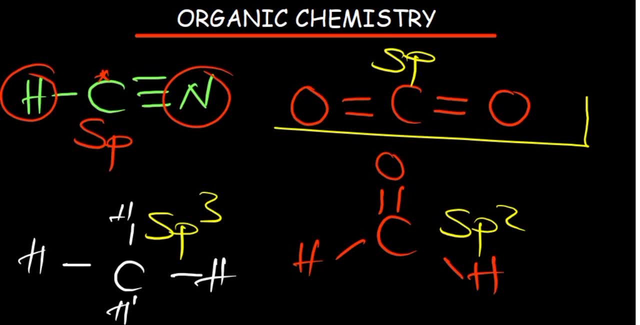 Two. So therefore we'll count the first connection as s and then the rest to be p. Okay, of course, the maximum is sp3.. And so carbon undergoes three different kinds of hybridization. And if you look at this other carbon here, if you try to count s, let the rest be p. 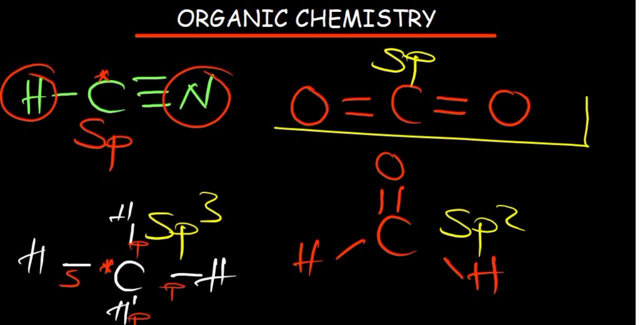 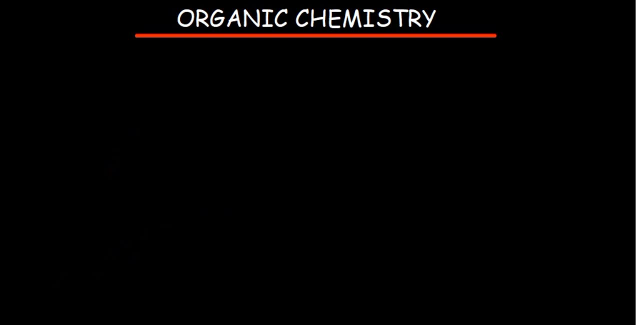 So you have s3.. You have sp3.. Of course, in the actual sense, this is not basically what it implies. Okay, So if we go back to our hybridization under chemical bonding, we realize that if we are to draw, of course we've talked about the electron configuration of our carbon atom, right? 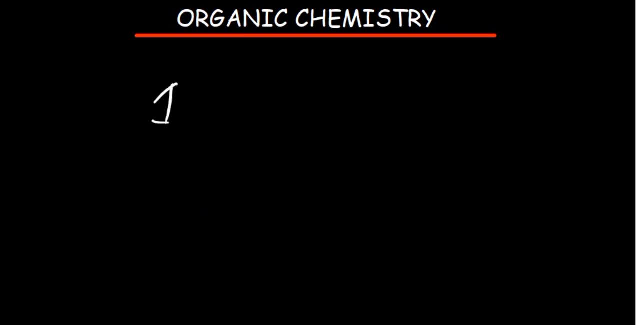 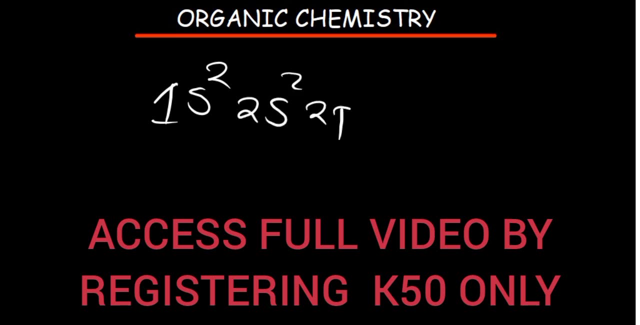 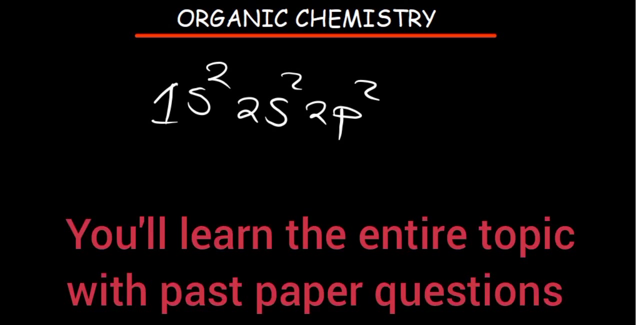 So what have we said? We've said the electron configuration is 1, right. So we said 1s2.. And then we said 2s2.. And then 2p2, right. So if we are to show this on our molecular orbital diagram, what we are seeing is something that is very interesting. 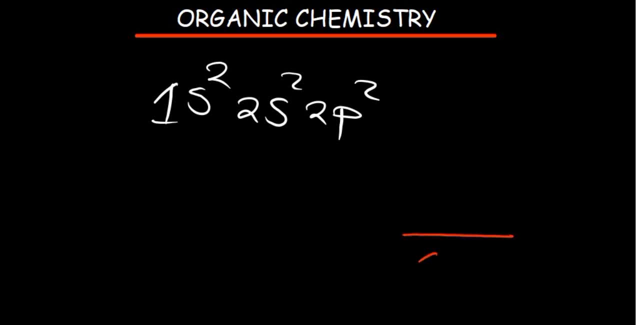 So we have our inner orbital, there 1s, which is adding two electrons, And then we have 2s as well, So I can show 2s somewhere there, So 2s, which has got two electrons as well. 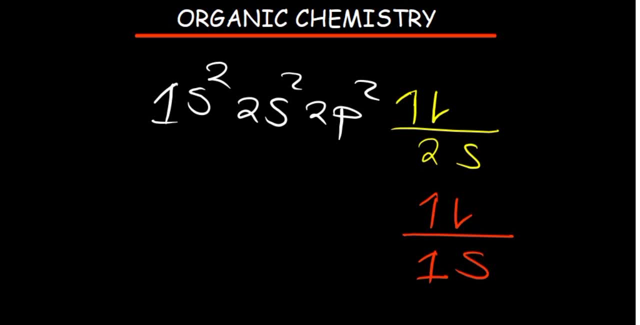 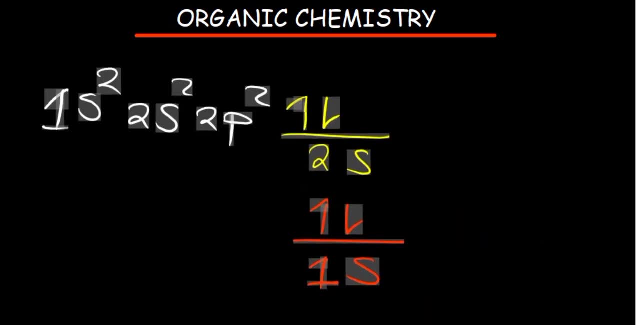 And then we can have the p orbitals. So let me just move this a bit, this side, so that we're able to see clearly. Okay, So, and then we have p orbitals. So p orbitals- we know that p has got is able to accommodate up to six electrons. 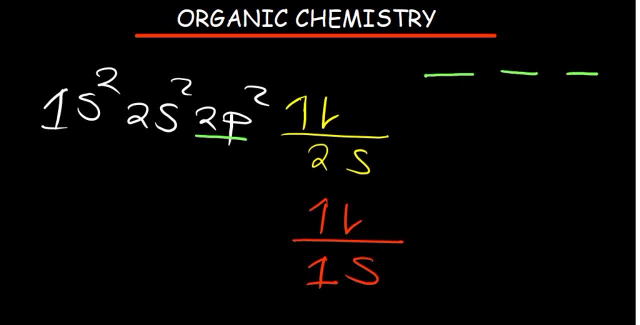 So I'll draw three different orbitals there. So that is our 2p And how many electrons are there. So we have only two electrons there. So looking at the number of electrons that we have, this gives us this diagram that we have here. 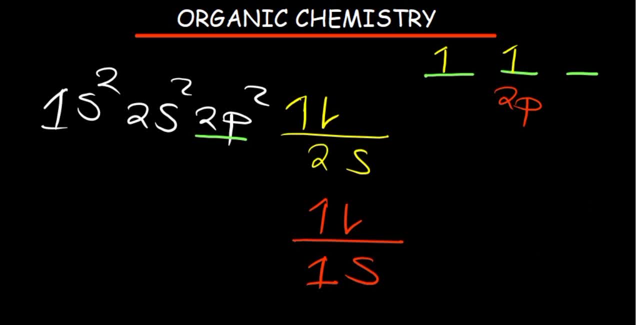 Now some funny, funny questions that they can give you. under organic chemistry, You need to write the excited state of the electron configuration, of the excited state of a carbon. So in the actual sense that we have is this is the basic electron configuration, or ground state electron configuration, of a carbon atom. 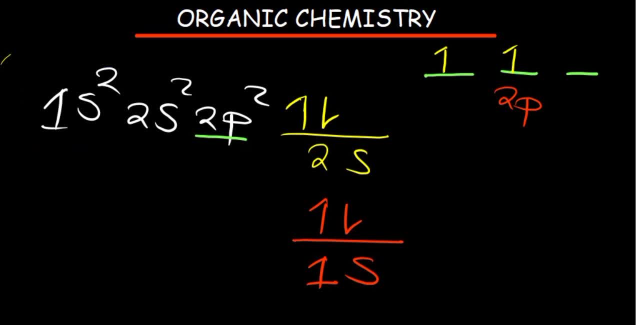 Now, what about in the excited state? So, in the excited state, what basically happens is this electron that you are seeing there is going to shift and go to that point there. So therefore, in the excited state, we expect that there will only be a single, so that electron will go there. 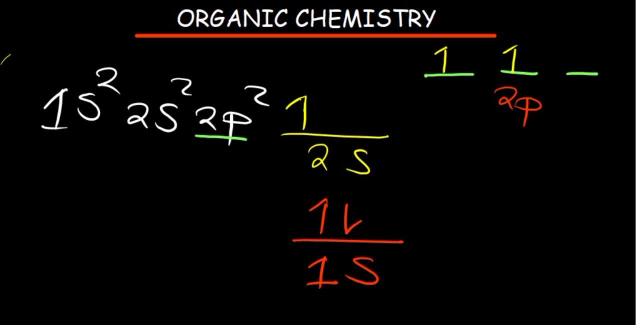 So there will only be a single electron in the 2s orbital. Okay, So now, this is what allows carbon to form up to how many bonds? Up to four bonds because of this semi-divide. Okay, Now, how is it possible that it is able to form up to three different kinds of hybridization? 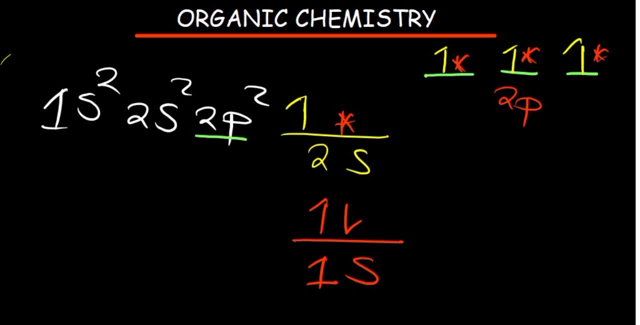 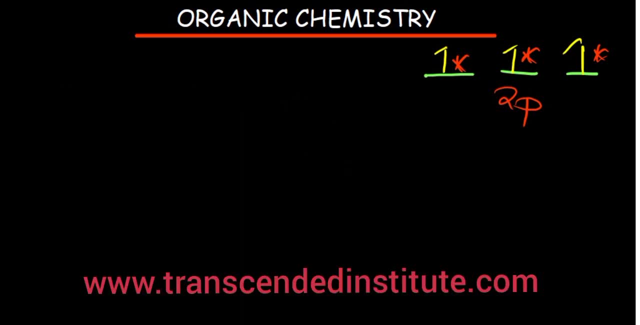 So I can show that as well. So I'll forget about what was down there And then we'll just focus on the outermost. So I'll drop the 2s a bit down so that we're able to see. Of course, take note that there is also 1s down there somewhere, down right. 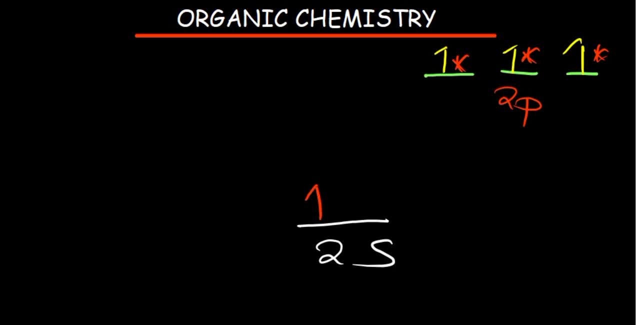 Very important. Okay, And of course I have not written the excited state configuration, electron configuration. So, in the actual sense, what we started with is we added 1s2 as our ground state electron configuration of our carbon atom, And this was 2p to the right. 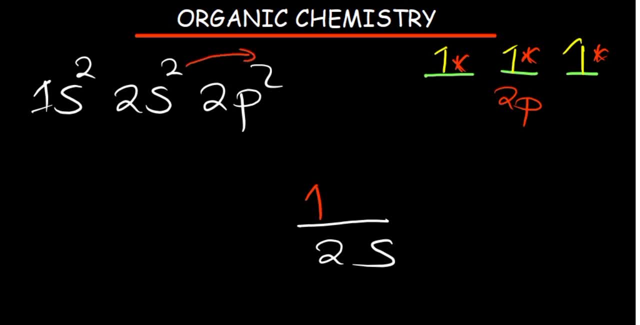 So what has happened is we've seen a shift of an electron to there. So in the excited state we expect we are going to have 1s2, 2s1, 2p3.. This is the excited state of a carbon atom. 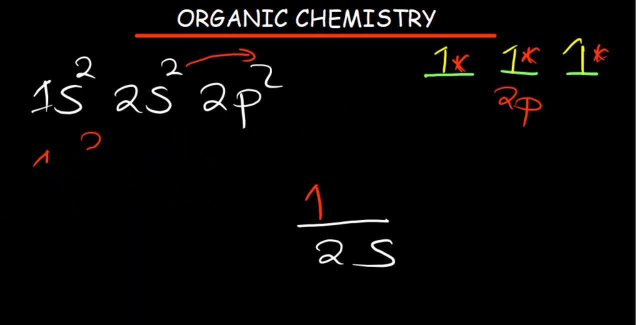 Okay, So it is reacting, It is in the excited state. Okay, So now what basically happens? So I'll start with, first of all, the sp3 hybridization. Well, we have carbon forming up to three, four different bonds, right? 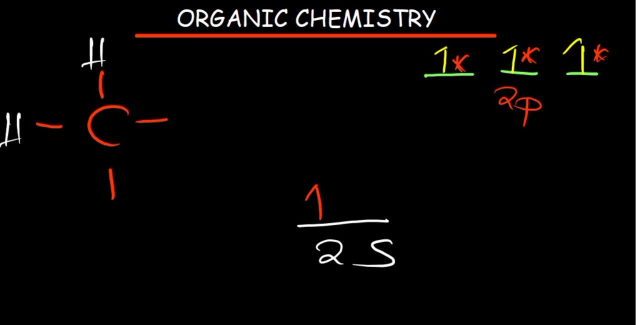 In methane, for example. How does that happen? So, basically, what happens is, since we are saying what is formed is an sp3 hybridized orbital In the actual sense, if you look at the diagram, what we would expect is we need to have four different what? 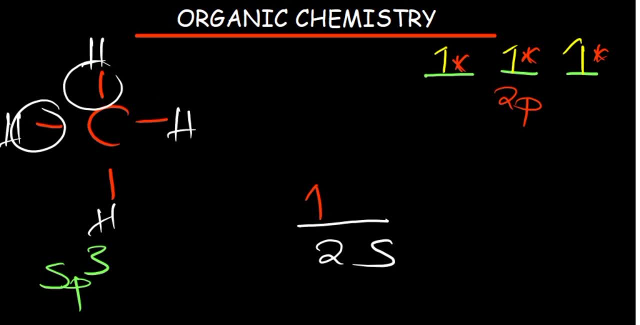 Four different orbitals because we have got four different atoms coming in. So what is going to happen? So what is going to happen is we're going to have, since it is saying, sp3 hybridized. And of course I gave you a simpler way of you identifying the kind of hybridization by first of all counting the first connection as s. 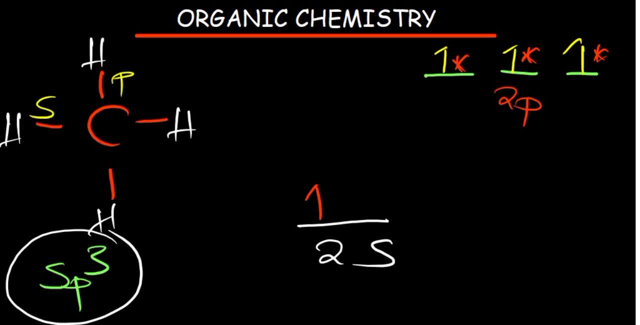 And then counting the rest to be p's. So that is the shortest way of you identifying. So, after you've identified, you're now convinced to say there is a combination of a single s orbital and three different p orbitals. So therefore, since we have three p orbitals, it implies that all these three p orbitals are going to be involved in the, in the bond formation. 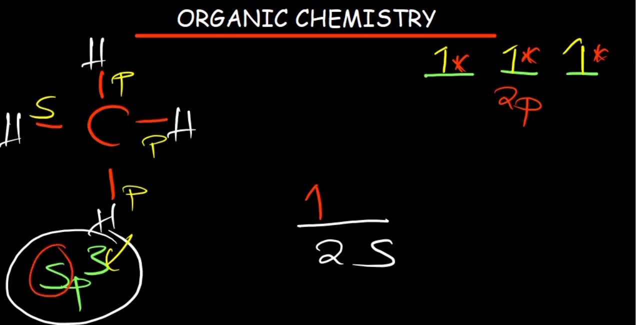 And then the s is also going to be involved And, of course, if you go back to a chemical bonding, what we know is hybridized orbitals have got the same energy, So we expect that We expect them to be closer to the p orbital, because it is 75%. what? 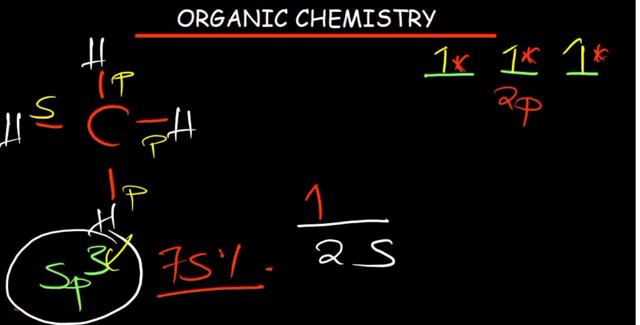 p. Okay, And then they just because, if you look at the total number of orbitals, we have four, So it's 75% if you look at three out of four. So therefore, they are going to have the same energy, but they're going to be closer to the p orbital. 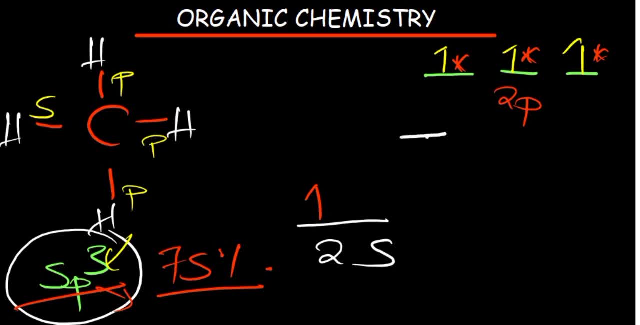 So I can show them somewhere there. and they're going to be four: One, two, three and four. So which of these four? So this four is the combination of this s orbital And those three p orbitals are giving us now what we call sp3 hybridized orbitals, right? 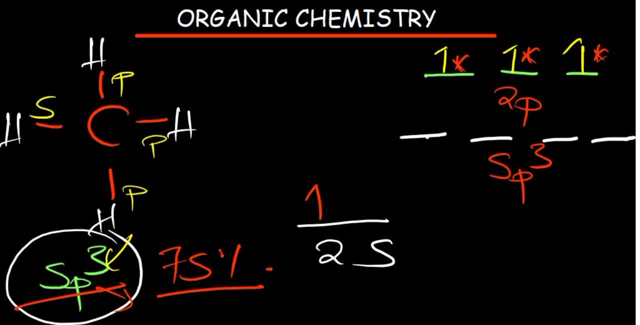 So we have four sp3 hybridized orbitals that are formed in such a case And of course, we are going to have how many electrons? Single electron each, So, and then this one is also going to be there as well. So what will basically happen is, this is the kind of orbital. 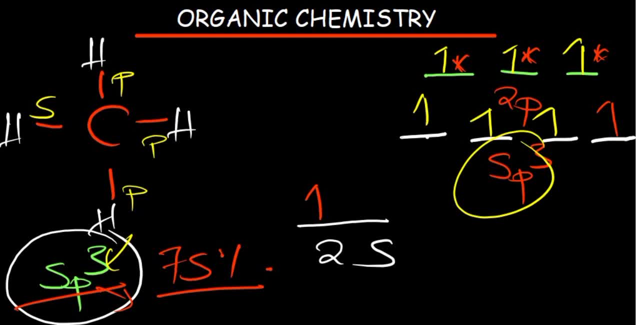 That is, these are the kind of orbitals that are going to basically take part in the bond formation with a single hydrogen atoms. So the hydrogen atoms are going to come with electrons there. So, in the actual sense, what we're looking at is an overlapping between the s orbital of each hydrogen atom, overlapping with a single sp3 hybridized orbital of the carbon atom. 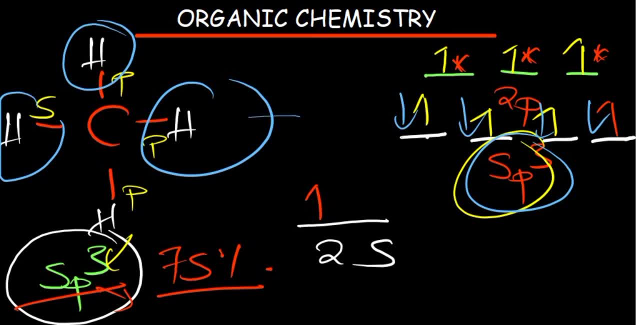 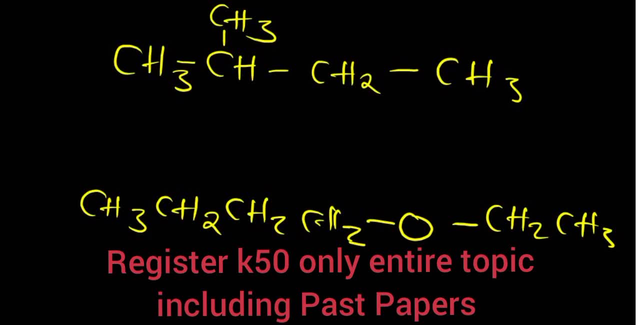 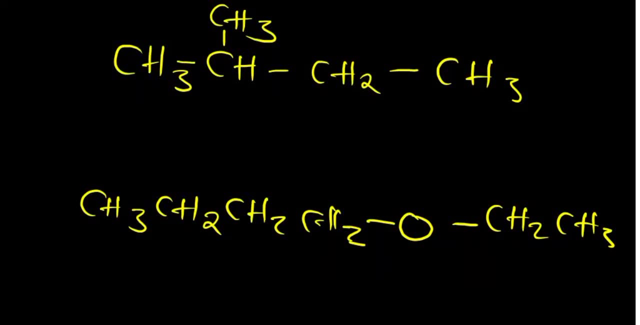 Okay, Interesting. Let's illustrate the other kind of hybridization. Okay, So if you wish to access the entire lesson, you can basically register using the link in the description. Otherwise, also learn how to go about this. So we call this UPAC. 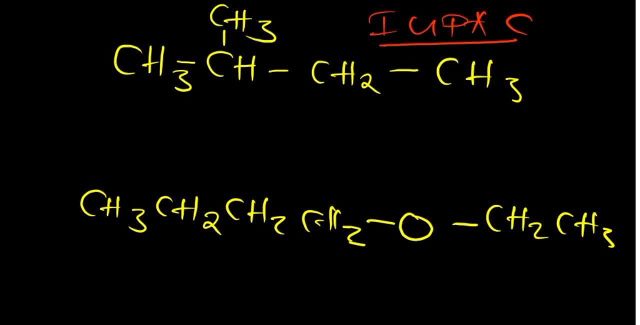 So UPAC nomenclature. What are the rules? Basically, that this union came up? Of course UPAC stands for International Union of Pure and Applied Chemistry, So it's a union that is in charge of on how to name the compound. 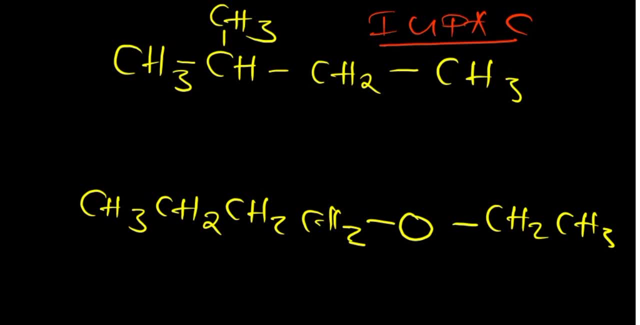 So we've got rules that we get to follow, So I'll introduce you to the rules using these two examples here. Okay, So each time you're trying to name a compound, you need to identify the longest chain of carbon atoms. Okay, 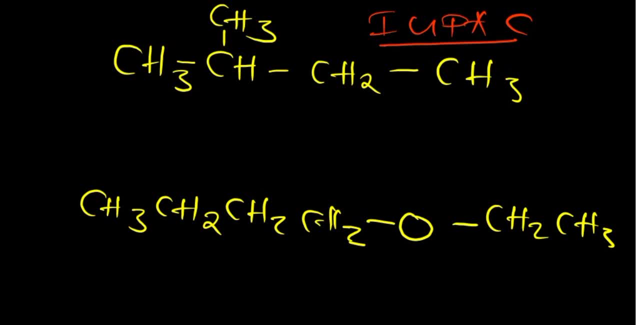 So in this case it is very easy for you to tell, because the horizontal one is obviously the longest one, right? So we have one, two, three and four. Okay, So you need to ask yourself a question to say what kind of an alkane has got four carbon atoms? 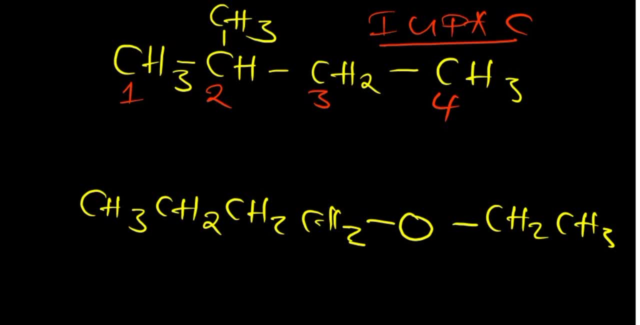 So of course you need to know the order. of course The first one is meth, And then we have earth, We have prop, And then we have bat, We have paint, So all the way up to ten, right. 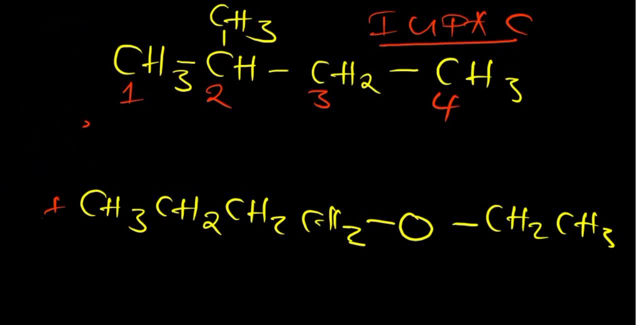 So in that video you have access to all that And, of course, number four, we are able to see that it's bat Being an alkane is butane right. Okay, So we also have what we call the substraints. 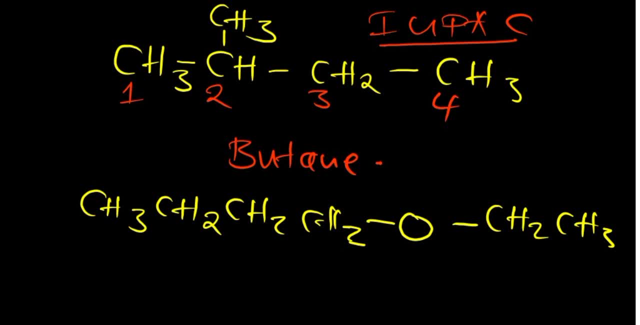 So now substraints basically are usually the other groups that attach to the main chain or the longest chain. So in this case we can clearly identify CH3 to be what To be a substraint. So what is a substraint? So basically, something attached to a parent of the longest chain of carbon atoms. 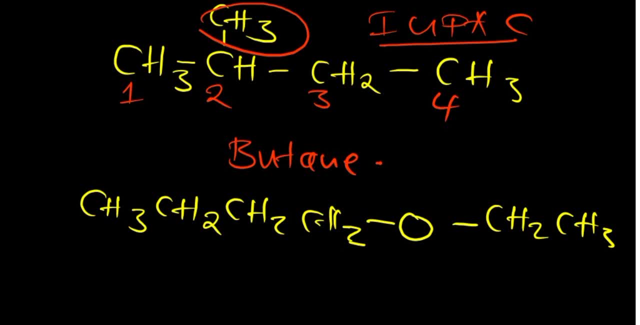 That's what we have Now. I also want you to know that we also have what we call alkyls. So alkyls, basically in a simple way, is just basically an alkane that has lost a hydrogen atom. So, for example, if you look at ethane, which is CH4, if it loses an hydrogen atom, it becomes CH3, which is going to remain. with what? 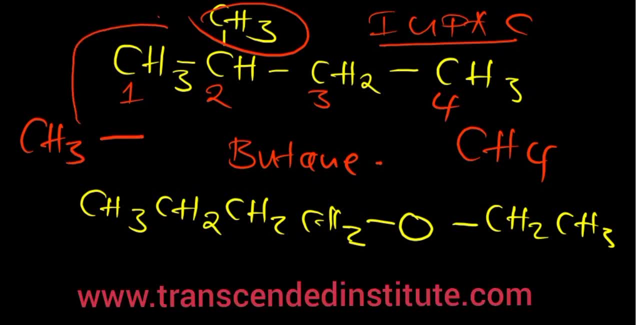 A bond there. So CH3 is what we are seeing as a substraint in our compound there. So the name changes from methan, which was ending with A, and E, from an alkane It will now become methyl. So we add YL to our prefix. that you are able to know from meth all the way up to decane, which is for number 10.. 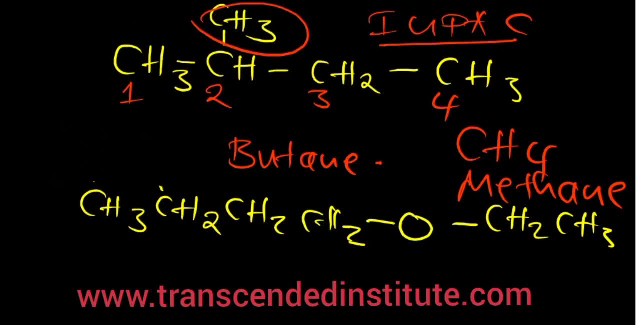 And then we need to also give it a position On which carbon is it joined, So somebody else may decide to start counting from the right hand side Where they will say, okay, one, two, three, four. This number says they are joined on carbon. 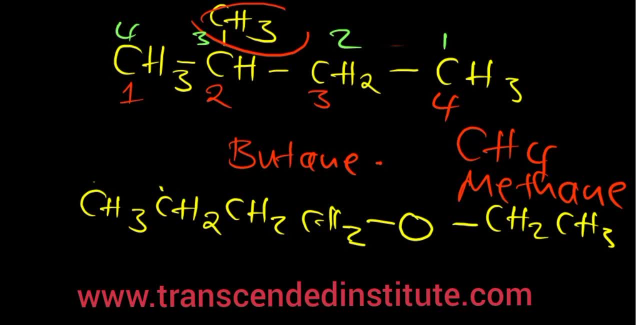 It is joined on carbon three. So therefore, I want you guys to understand that we need to go for the one that is giving it a lower positioning, So in this case, we can say that our methyl is joined on carbon number two. Okay, 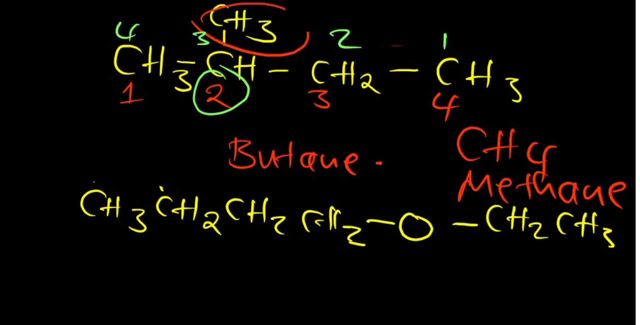 So therefore our name becomes 2-methyl. So the substraints, basically, are considered to be the prefix, And then the parent structure or the parent name, basically is the suffix, which is towards the end. Okay, So what if I decided to add an extra methyl somewhere there? 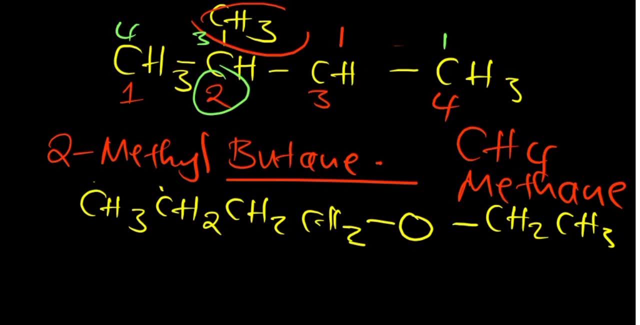 And then we can remove a two there so that it becomes CH3 here, So that now becomes: we have now two methyl groups. Now, on what position is the other one? It is on position three. So we can say, since there are two, we can just say di. 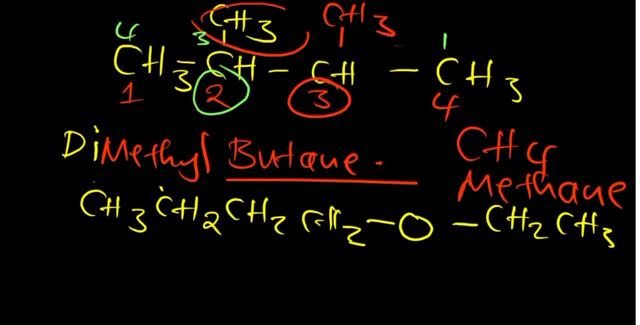 So di is a prefix that we're going to use for two. So we have di tri tetra and so on and so forth. So in this case it's di-methyl. On what position are they? So we'll say 2,3-. 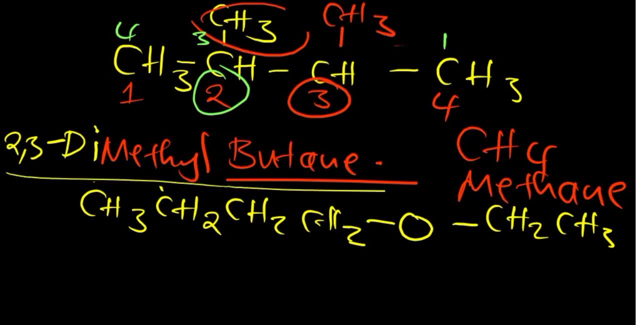 So that is how you name it in such a case. So there are many, many more things that we get to name. There are a lot of rules that are supposed to be introduced. What if you have other substraints? Substraints like alcohols, things like a fuse and many, many more? 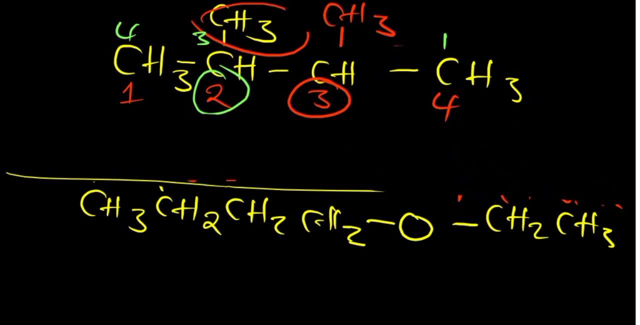 So all those things are going to be covered in our topic. So just access the course Register for the course. You have access to all that. And, of course, I would like to talk about the last one. So this is an example of what we call an ether. 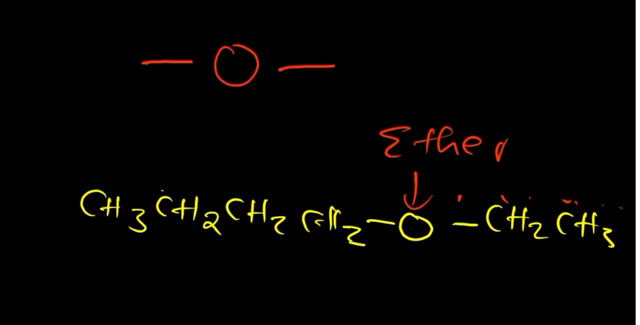 Whenever you see an oxygen with two bonds, so that is an ether right. So if you look at this side, how many bonds, how many carbon atoms do we have? One, two, three, four. So what kind of an alkane is that? 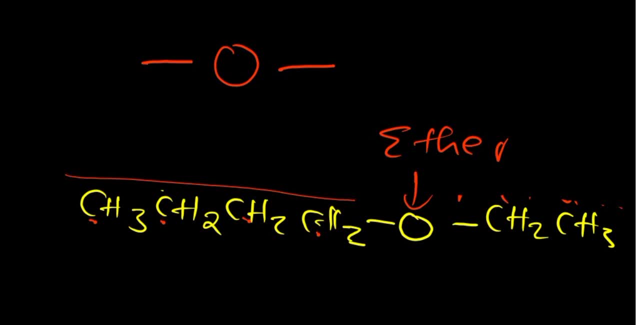 It's butane, right, So it's butane. Now, in this case, we can clearly see that this is a butane that has lost a hydrogen atom, So we'll consider it to be butyl. So we have butyl. 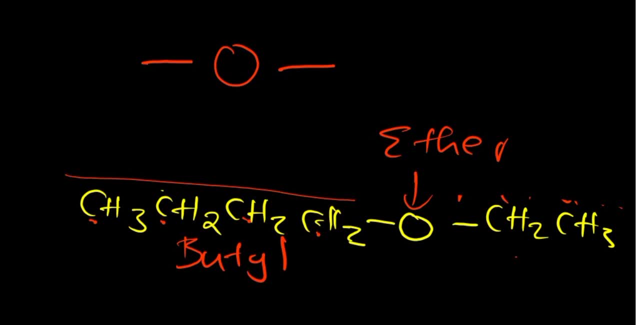 And then the other side, we have got two. So that is ethyl And then this is an ether. So basically, how do we get to name it? So, from what we have come up with the name, the common name can be based on the same. 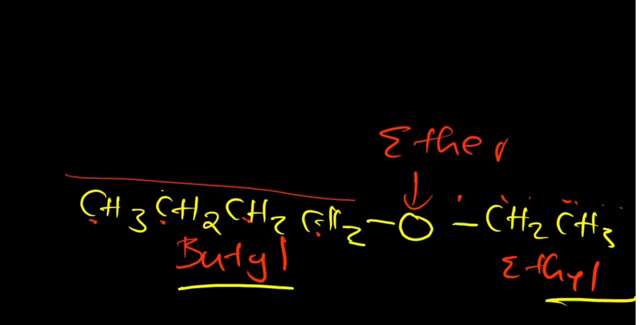 We'll alphabetize these two guys. The suffix is going to be ether. So we have butyl ethyl ether, So that is a common name. That's the common name of that ether. Now we also have the UPAC name. 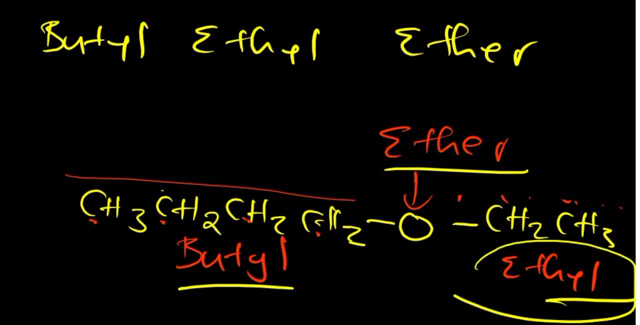 So the UPAC name tells us to say that you go for the shortest one. The shortest one is going to be the prefix, And then you need to add OXY, So the ethyl becomes ethoxy, And then the longest one consider it to be an alkane. 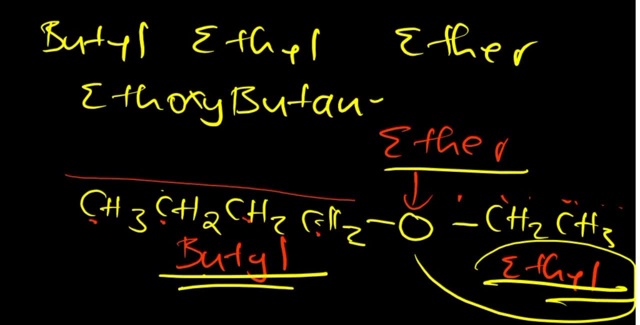 So it will be ethoxybutane, So that is the UPAC name of this kind of an ether. So all those are going to be covered in our course- I'm sure you don't want to miss it out- And of course, in our course, many other more things that we're going to cover will include 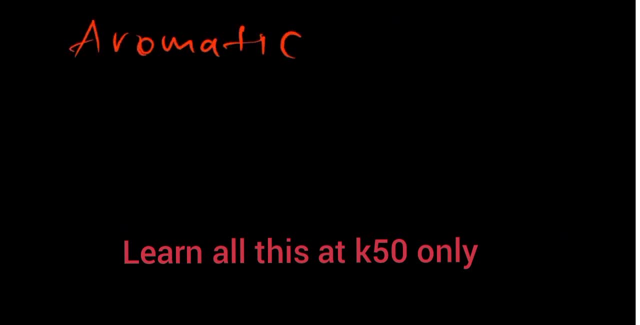 aromatic compounds like benzene, And then we'll also cover things like cyclic compounds. We'll talk about the reactions of alkanes, alkynes, alkalines and many other more compounds, Of course not forgetting substitution reactions, free radical reactions. 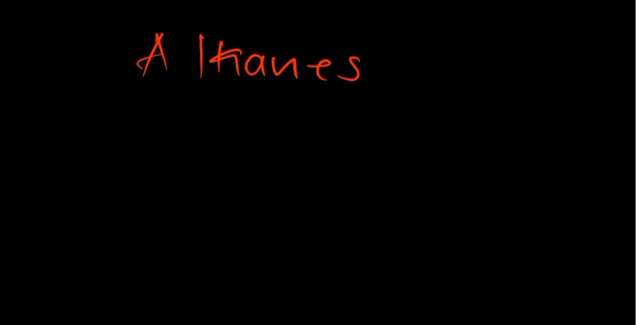 value structures. Now we get to come up with escalator structures. So the entire topic Organic Chemistry is going to be covered And, of course, we'll look at past paper questions together with the past tutorial sheet questions and the current ones that are yet to come out. 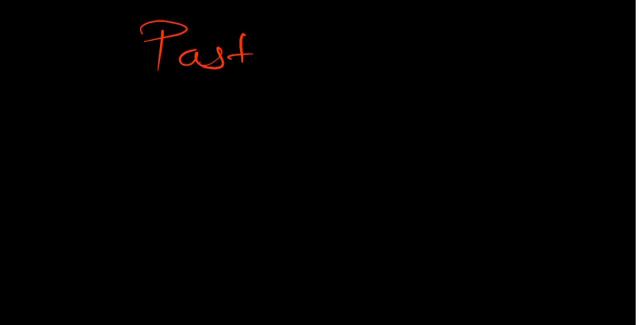 to make sure that your journey through Organic Chemistry is going to be very smooth. So to access the entire topic, it's just basically 50 kwacha. Or if you want to join the entire chemistry course and access all the other topics from the chemistry is 100 kwacha subscription per month. 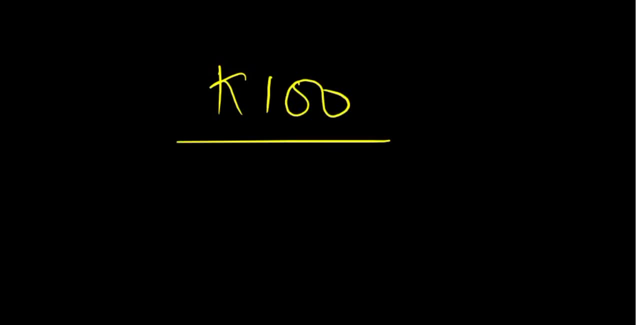 So thank you very much for making it to the end of the video. Feel free to share the video with your friends who would want to learn Organic Chemistry the smart way. Of course, we need to enjoy this, not just mastering. It's very simple. 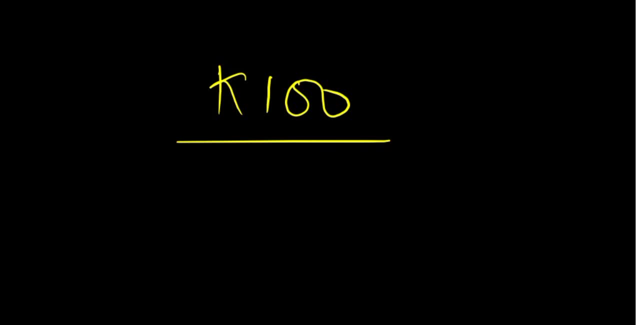 And I'll challenge you guys with a lot of questions throughout the entire course.